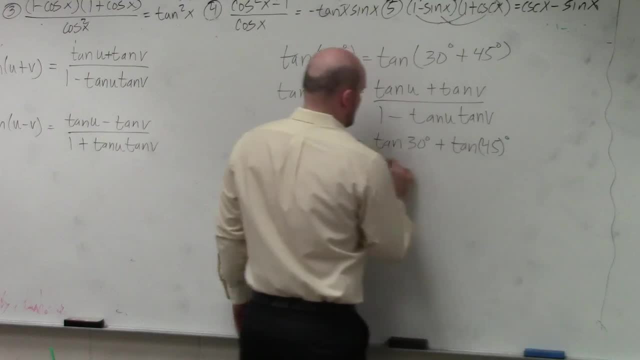 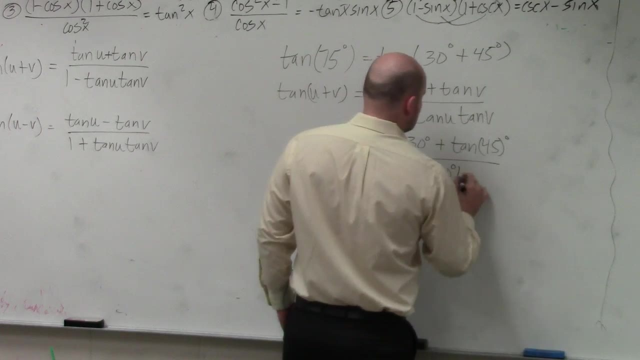 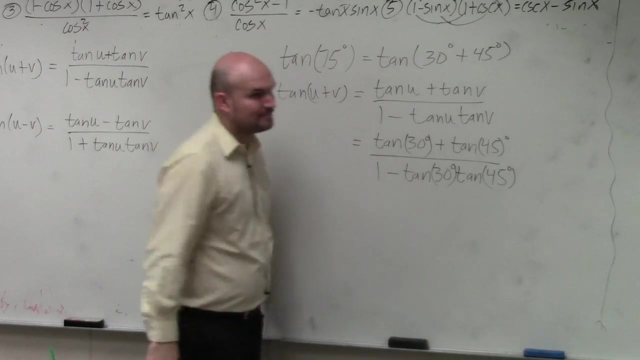 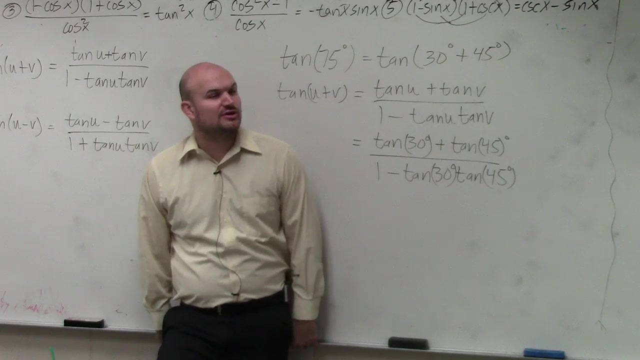 the tangent of 45 degrees, All over 1, minus the tangent of 30 degrees times the tangent of 45 degrees. OK, Now, the reason why we did our worksheet is: Josh, you had pi over 3, right, Remember tangent. 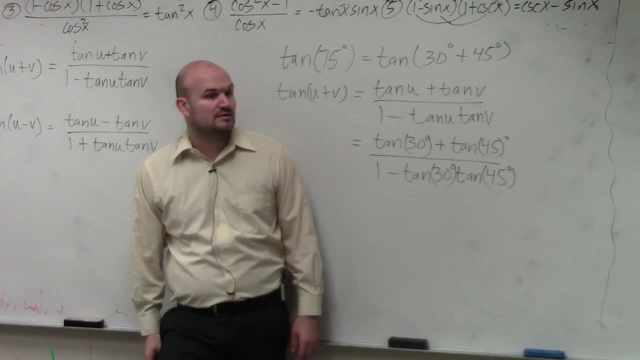 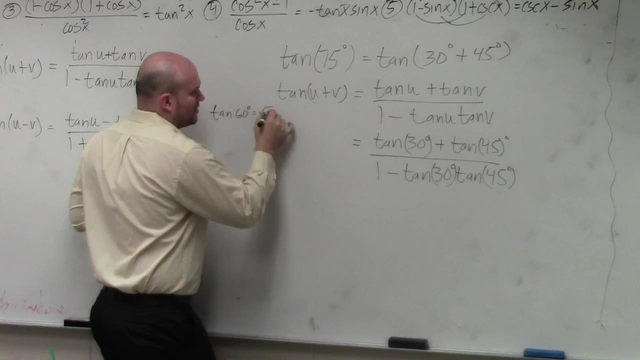 of pi over 3, the one you corrected me on That. simplified to what Square root of 3.. So we know that the tangent of pi over 3 is 60 degrees. right, Is square root of 3.. So therefore, the tangent of 30 degrees, which was also a problem on that. 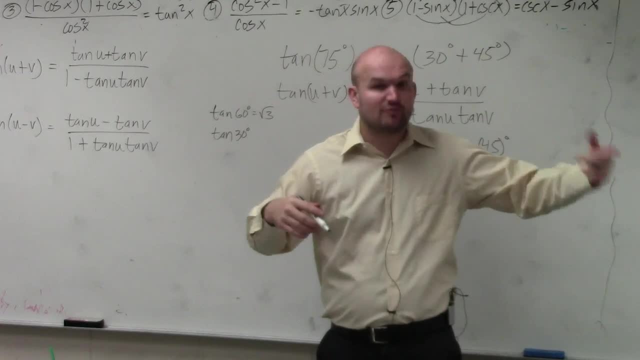 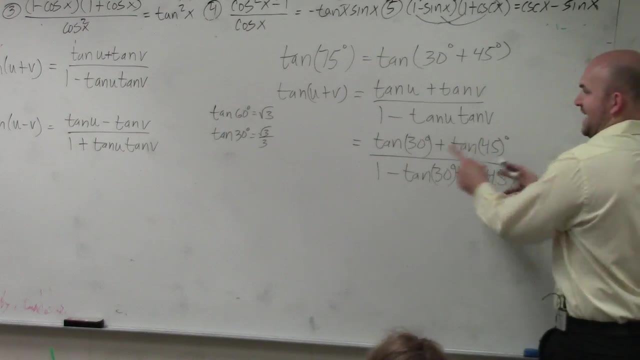 quiz that I gave you at the beginning of the class period, that one was square root of 3 over 3, correct? So you guys are going to need to remember those because a lot of times I'm going to be asking you what the tangent of 30 degrees, tangent of 60 degrees, tangent. 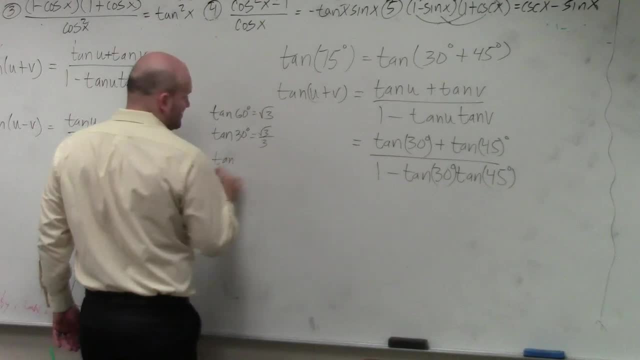 of 45 degrees. Well, tangent of 45 degrees. that one's the easiest right, Because that's the same number, right? So square root of 2 over 2 over square root of 2 over 2.. So that's. 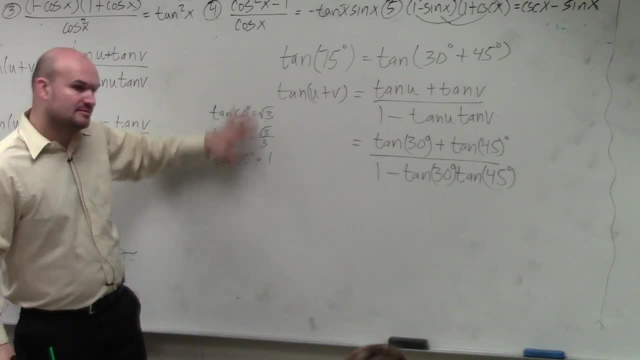 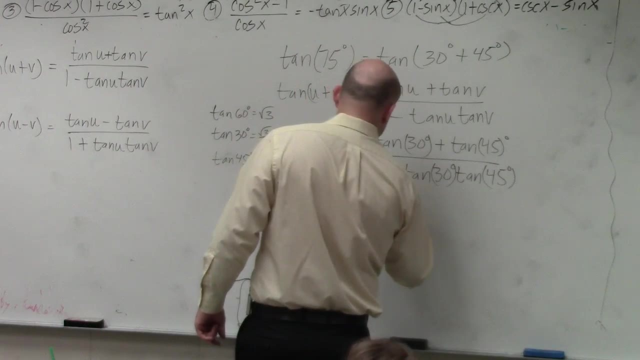 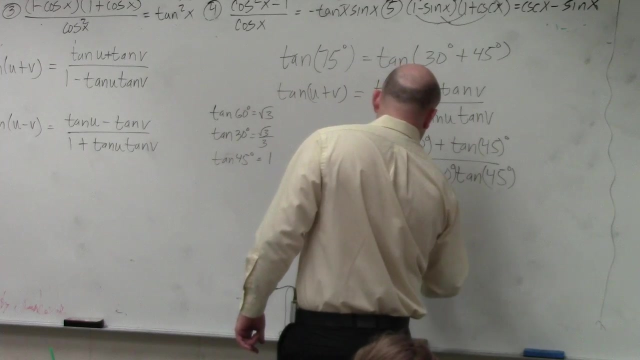 just 1.. So you guys want to make sure you remember these real easily. These are obviously only for the fourth quadrant. So tangent of 30 degrees is square root of 3 over 3 plus. tangent of 45 degrees is 1 over 1 minus square root of 3 over 3 times 1.. 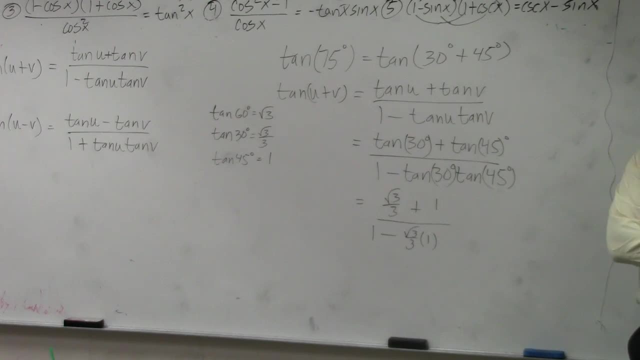 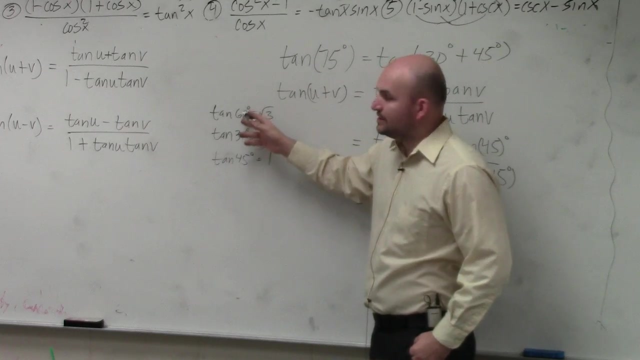 So everybody see what I did. Huh, Yeah, you can solve for it, I mean, but you're going to get the same answer. I'm just saying I didn't say you memorize these. You should already know these. You should know what the tangent of 60 degrees is Is tangent of 60. 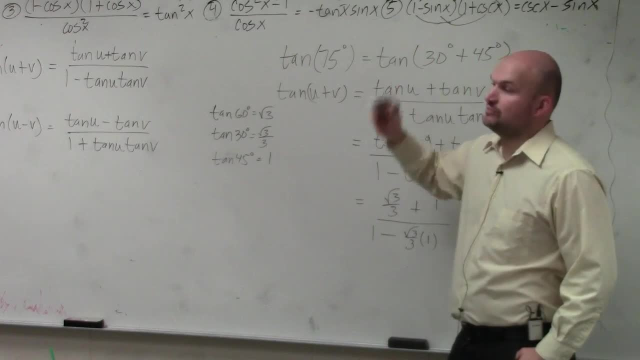 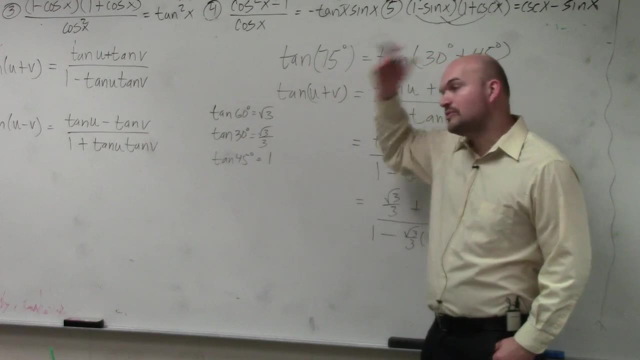 degrees is the coordinate point 1, half comma. square root of 3 over 2.. Do y over x. I'm just saying you don't need to do the math every time. You should start noticing the pattern that that's always going to be that square root of 3.. 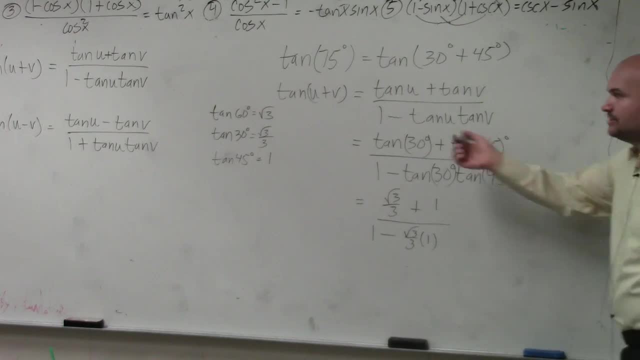 I'm just saying: recognize those patterns. for that I mean you can do the unit circle just like you did in your quiz. You'll get the same answers. I'm just saying to kind of speed it up because you can see how quickly I evaluated for all this right. 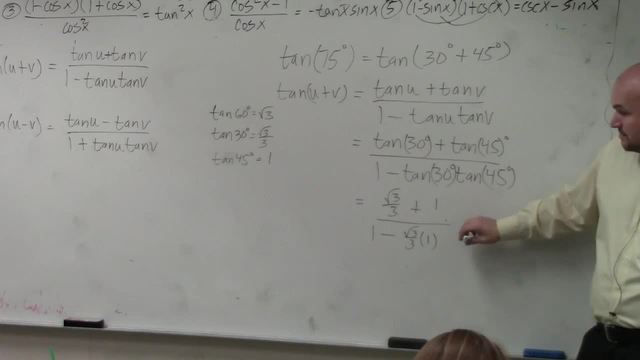 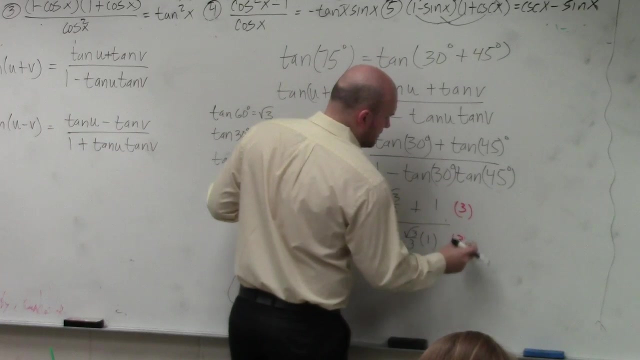 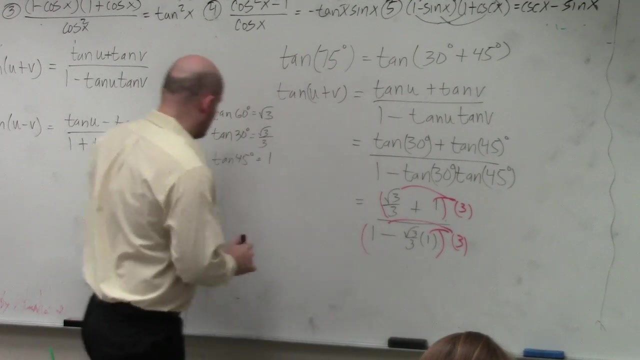 Now, this is really not technically simplified form, So the first thing I would do is: I see there's fractions in the numerator and the denominator. The first thing that I would do is multiply by 3 on the numerator and the denominator. Notice that these are binomials. So I'm actually going to have to continue my work over here. 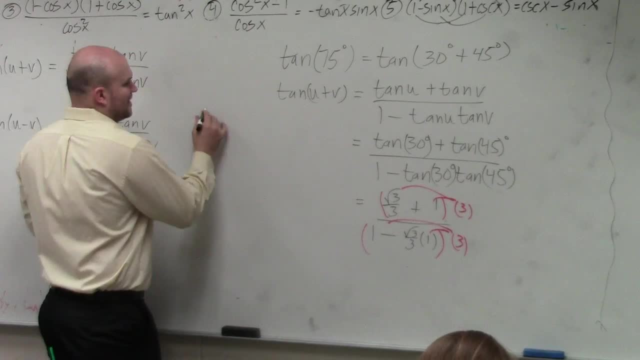 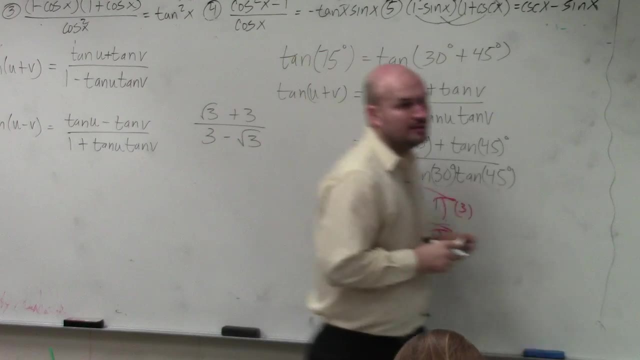 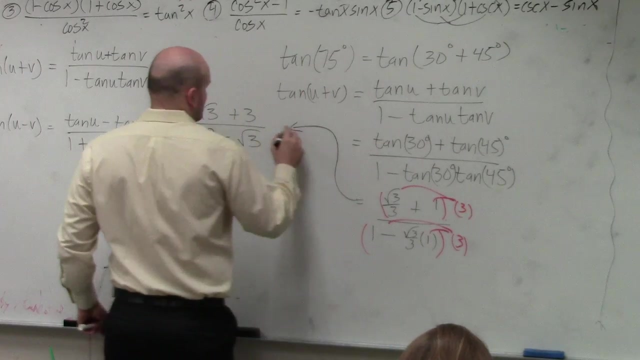 because this takes a little bit of work. So I have square root of 3 plus 3 over 3, minus the square root of 3.. Correct, And actually what we'll learn. would everybody agree this? 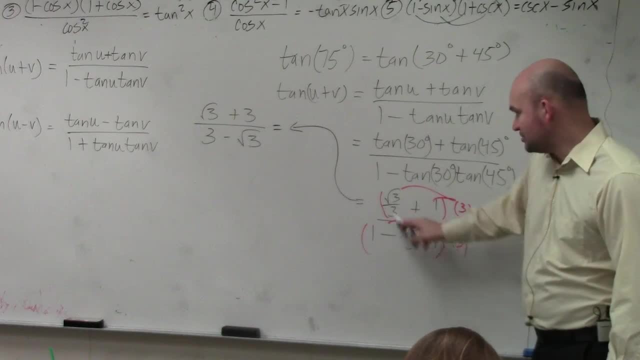 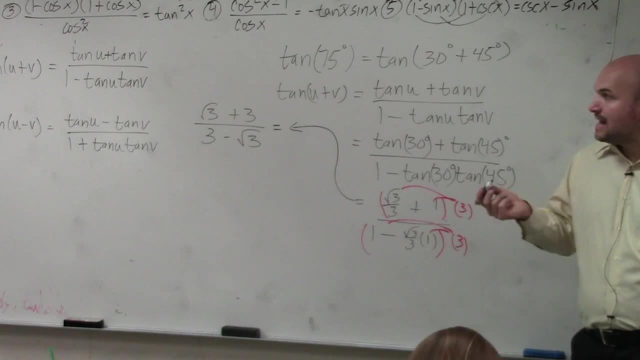 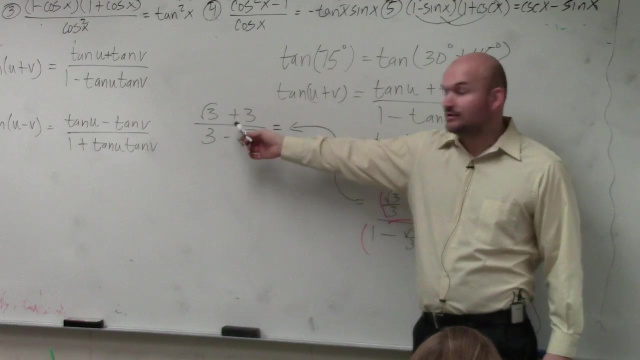 I'm multiplying the top and the bottom by 3 to get rid of these fractions, So I had to put them in parentheses to make sure I reminded myself to apply distributive property. Now, what I'm teaching in algebra 2 right now is when you have a radical expression divided. 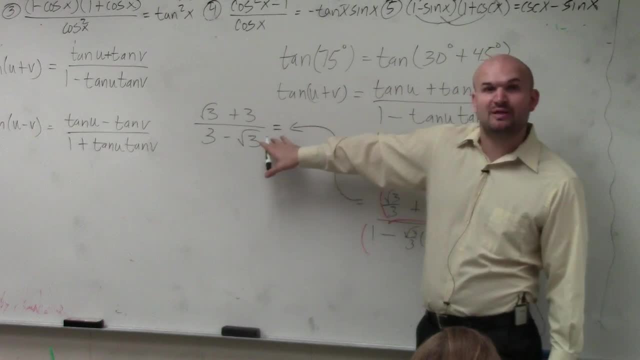 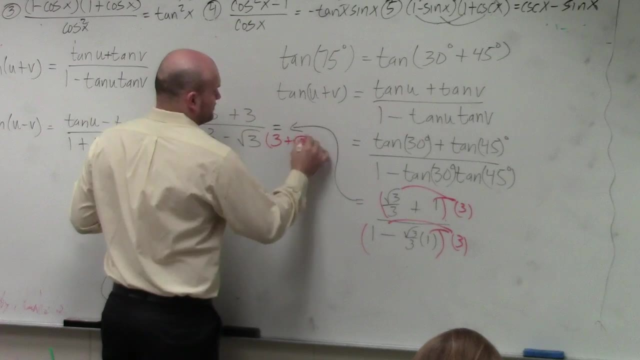 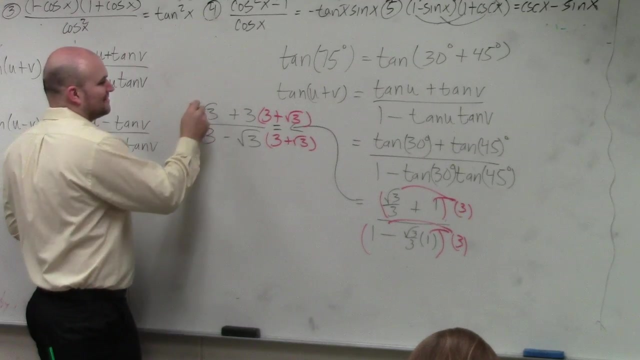 by another radical expression. we don't want to leave the radical in the denominator, so we rationalize the denominator by multiplying by its conjugate. That's why nobody likes doing the tangent problems So well. these are going to be irrational and complex. 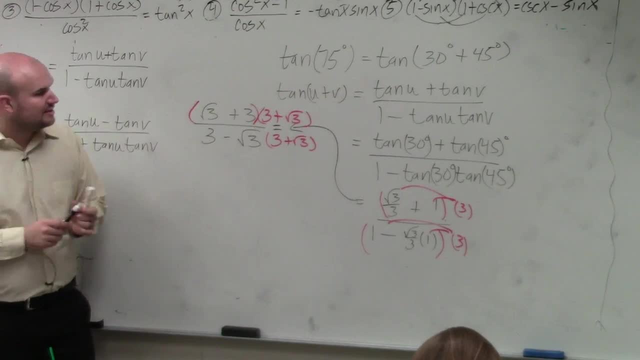 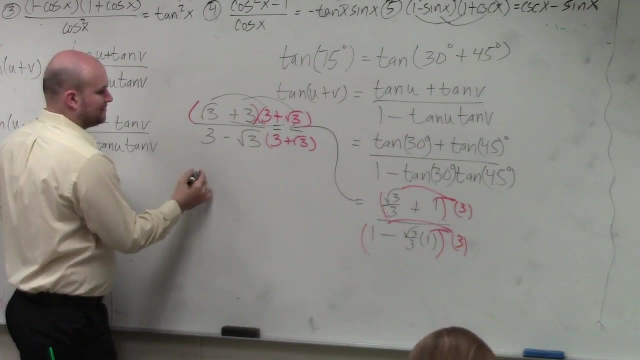 So this is racked to this positive, You're going to be multiplying by a complex conjugate. So here, all you're doing, basically, guys, is applying FOIL. This isn't anything that's crazy or new for you. The bottom your middle terms will cancel out. 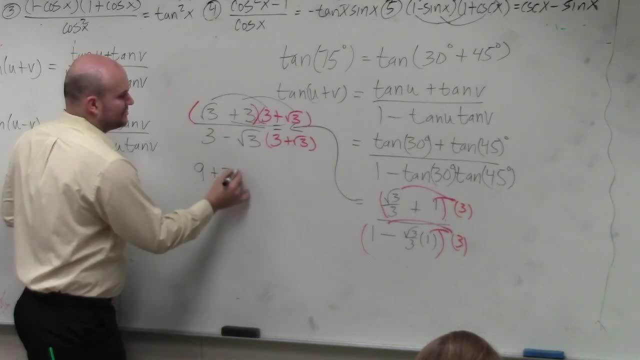 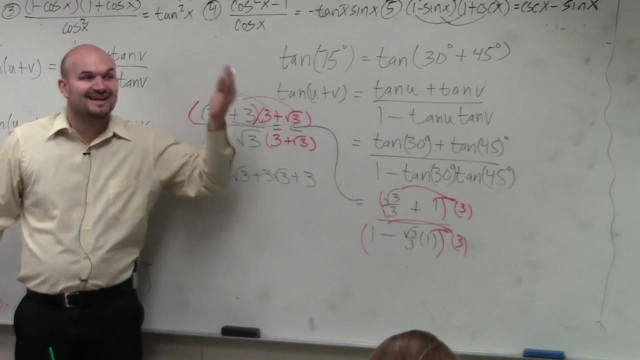 which I'll do two examples of. So we'll have 9 plus 3, square root of 3 plus 3, square root of 3 plus 3, because what's the square root of 3 times the square root of 3 is square root of. 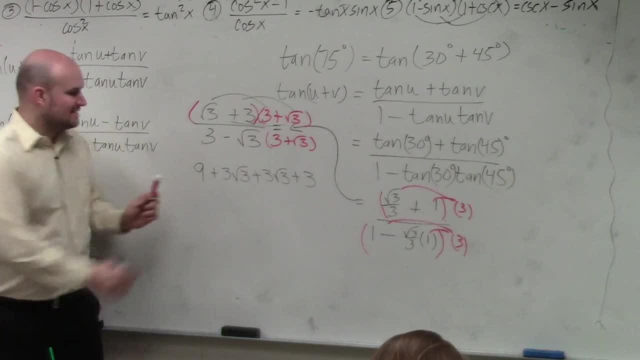 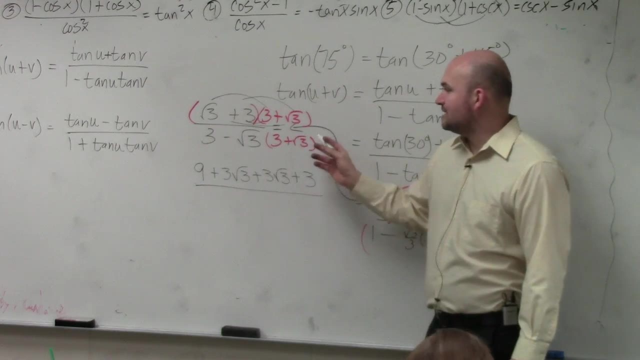 9.. And the square root of 9 is 3.. So therefore, that's there. And then the denominator. what's nice about multiplying a denominator by its conjugate is it becomes the difference of two squares. The middle terms are going to divide out. 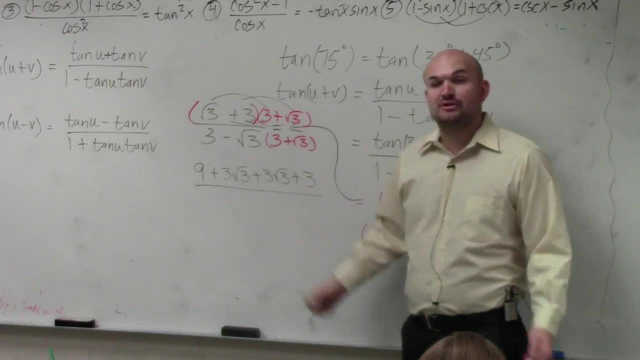 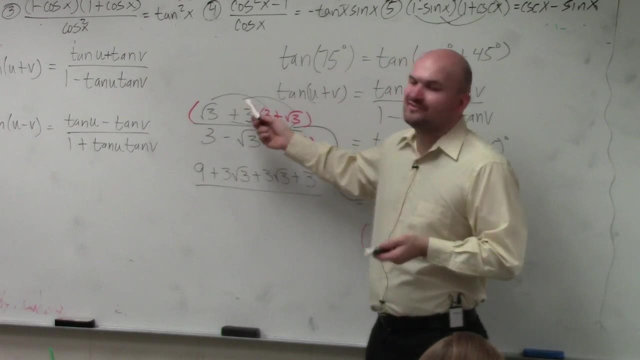 Where here the middle terms are going to add together Here the difference of two squares. the middle terms are going to subtract to 0.. How do you get 9 to the first square root of 3? I kind of switch them around. 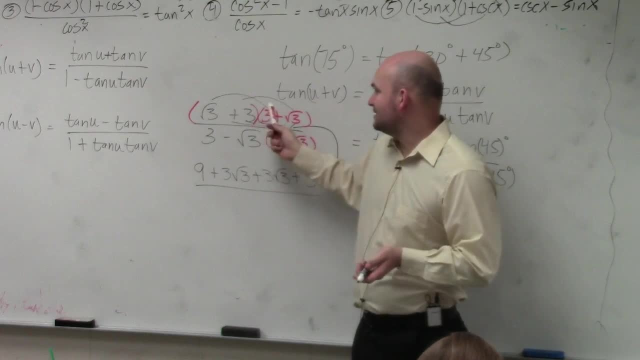 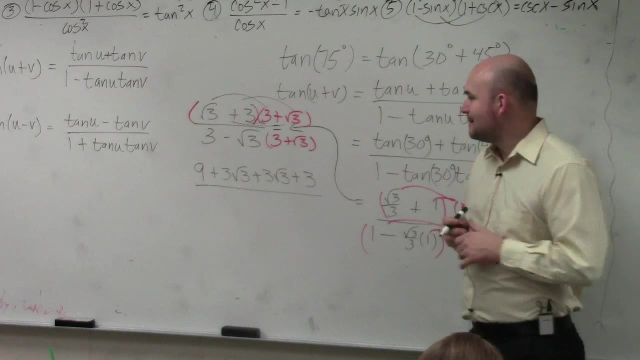 Yeah, I didn't really do FOIL, I just did 3 times 3 is 9.. And then I did 3 times square root of 3, 3 times square root of 3.. So yeah, I kind of switch them around in my head. 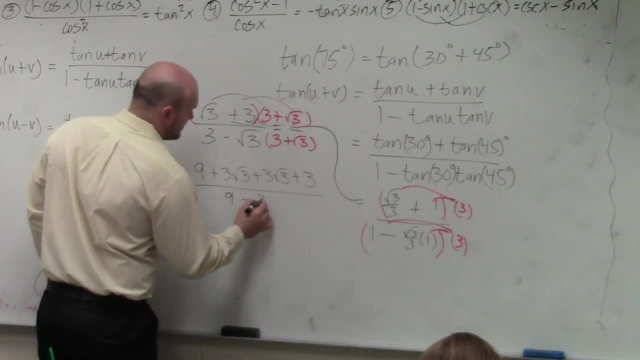 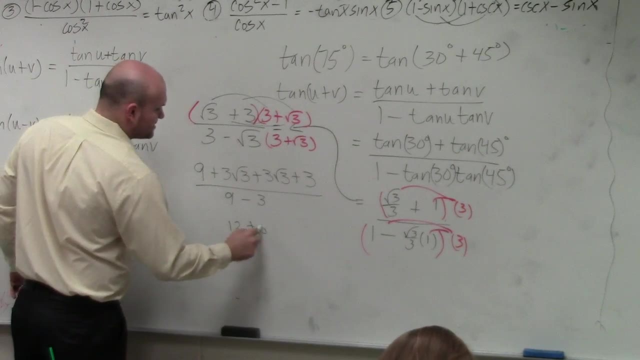 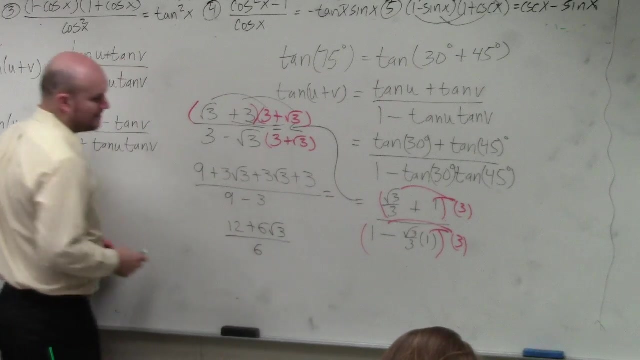 So then, over here, though, we'll have 9 minus 3.. Now we just simplify our answers: 9 plus 3 is 12. 12. 12. This becomes plus 6, plus 6, square root of 3, all over 6.. 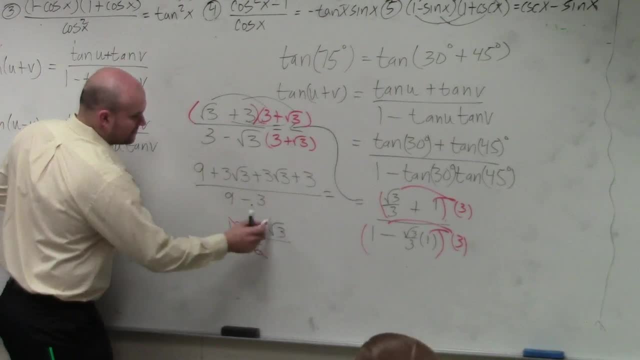 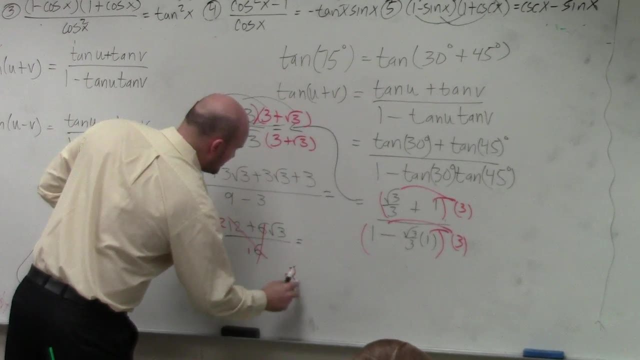 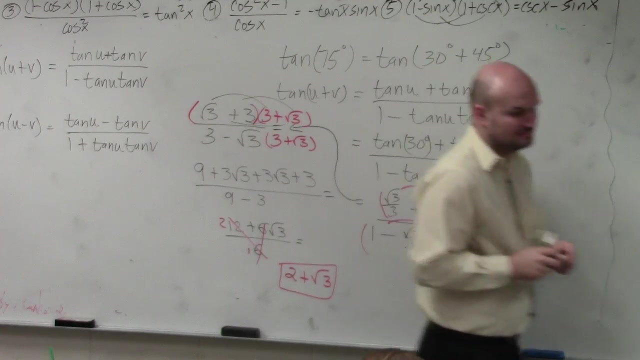 And then this 6 divides into both of these. So therefore, your final answer is 2 plus square root of 3.. And that's the answer that would show up on the test. So, yes, you have the formula which is given to you. 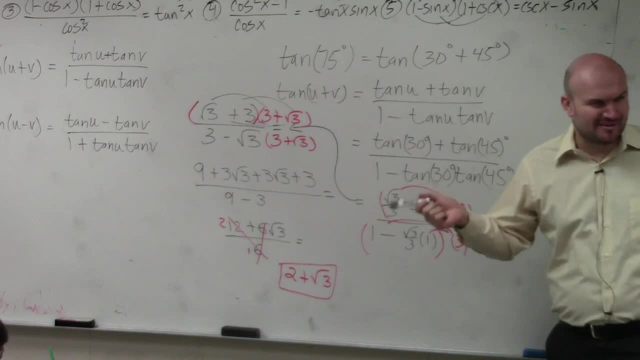 Yes, you have to evaluate. Do you guys remember telling me at the beginning of the year? I said, hey, you're going to have to evaluate for these functions like this. It's just going to be one little speck of a problem. 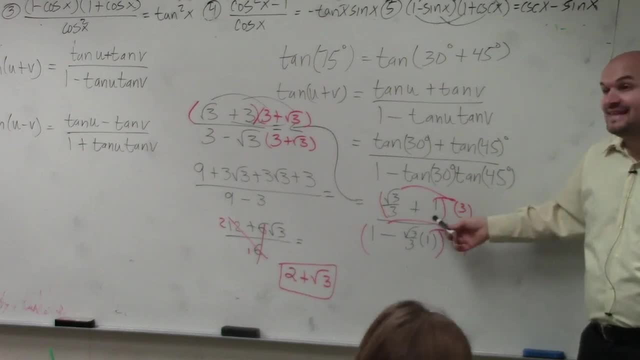 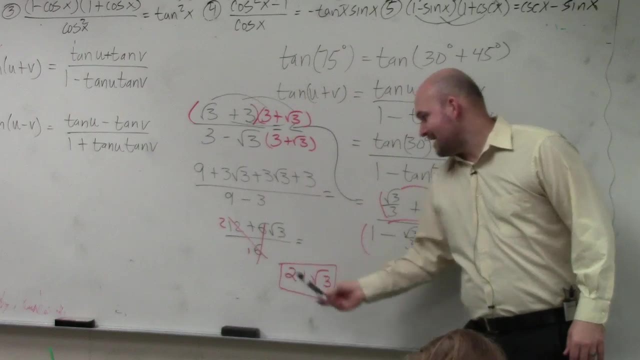 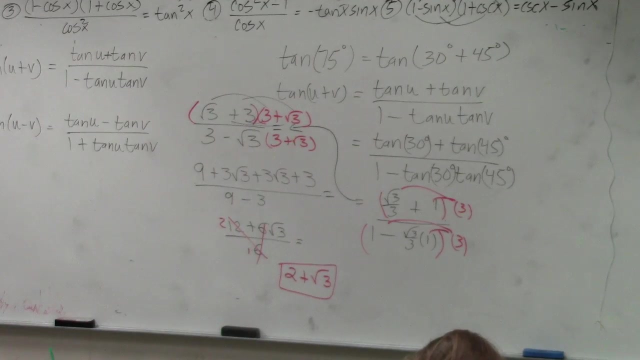 So you plug in your problems, You evaluate, Then we go back to knowing our algebra too. Getting rid of fractions, Rationalizing the denominator, Simplifying: That is your answer. These are great problems because they bring together like everything that we've been talking about so far. I mean, this is like huge. 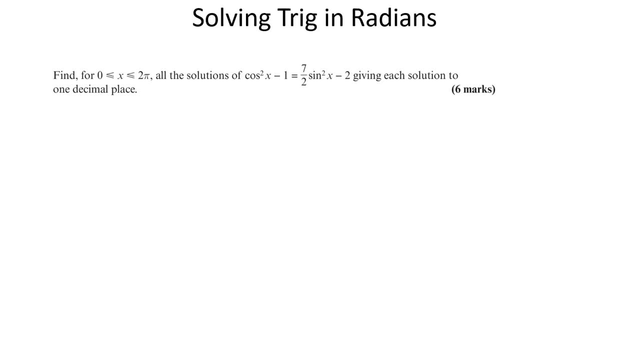 Hello, and this time we're looking at solving trigonometric equations, but doing it in radians. But that's not really any different to doing it in degrees. The process is the same, it's just that the range has the values in radians and, of course, our answers will be in radians. 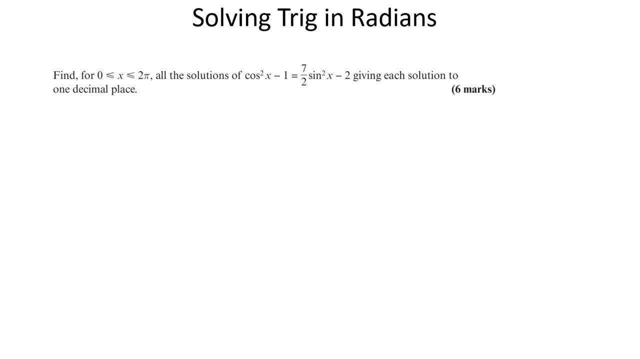 We're still going to use trigonometric jiggery-pokery to make this solvable, and then we're still going to use a cast diagram, or as I refer to it all students talk crap to look at the other values.